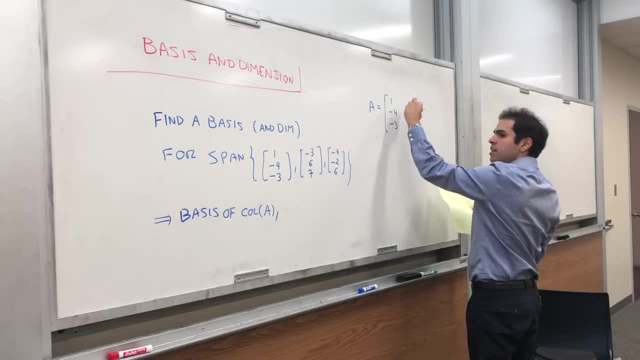 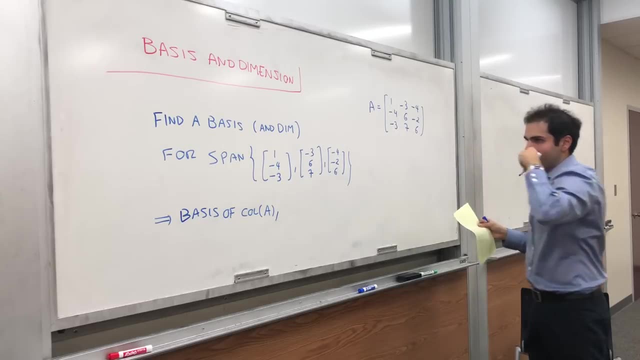 A is 1 minus 4 minus 3 minus 3, 6, 7 and minus 4 minus 2, 6.. Why is that? That's precisely by definition of the column space. The column space is just the span of the columns. 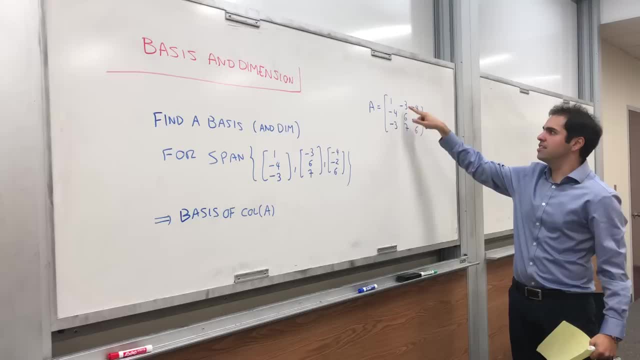 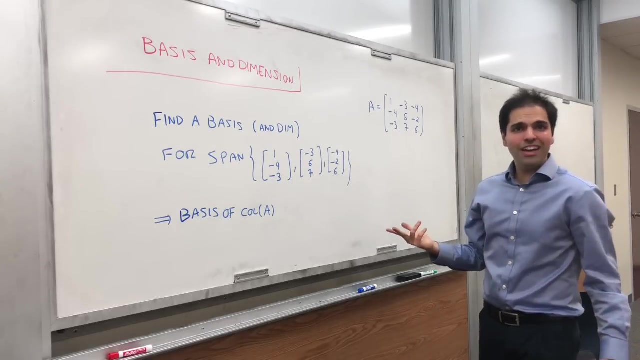 of A. Here the columns are 1 minus 4 minus 3 minus 3, 6, 7 minus 4 minus 2, 6. And if you take the span of this, you precisely get the span of those three vectors. Okay, how can you find a basis for the? 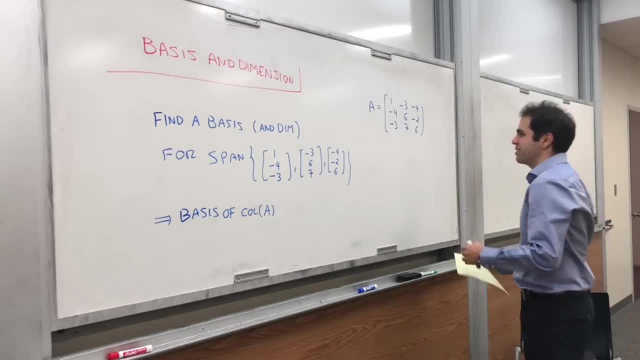 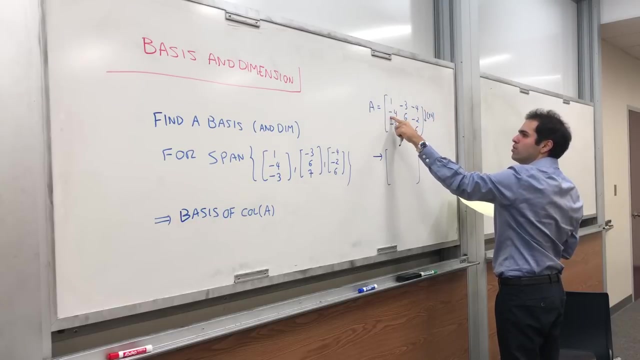 column space. As usual, you just rewrite it Now, a very useful technique. It's a nice thing about linear algebra: If you don't know how to solve a problem, just where we do this and it should give you the answer. So then let's add four times the first row to the 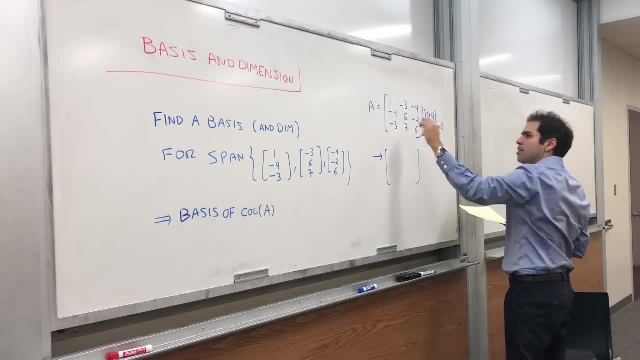 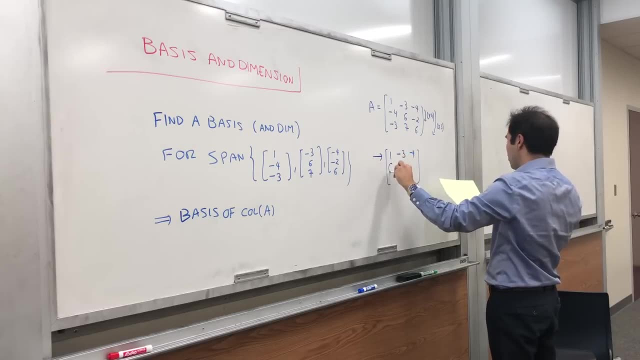 second row and three times the first row to the third row. then you get 1 minus 3 minus 4, and then 0, let's see minus 6 and minus 18.. And here you get 0, and then minus 9 plus 7,, minus 2, and minus 12 plus 6,, so minus 6.. 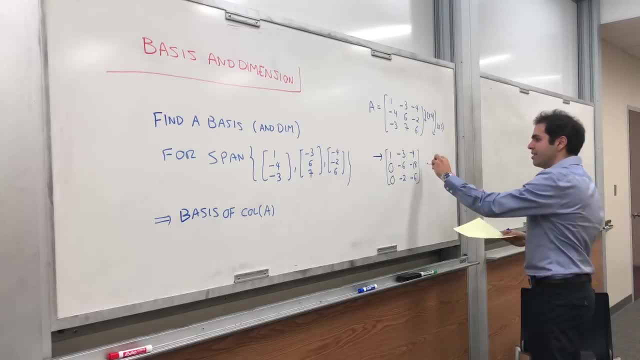 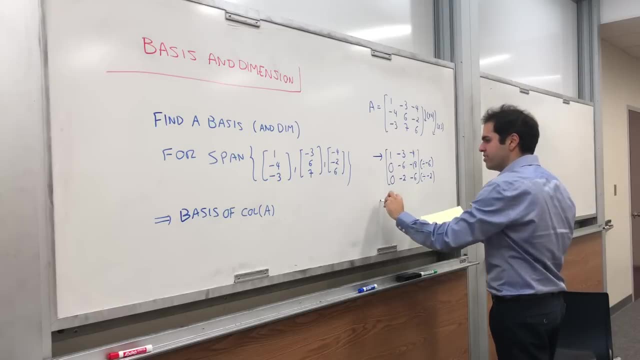 Before we continue, let's just simplify this a bit. Notice: the second row is divisible by minus 6, and the third row is divisible by minus 2.. So we get 1 minus 3 minus 4, 0, 1, 3, 0, 1, 3.. 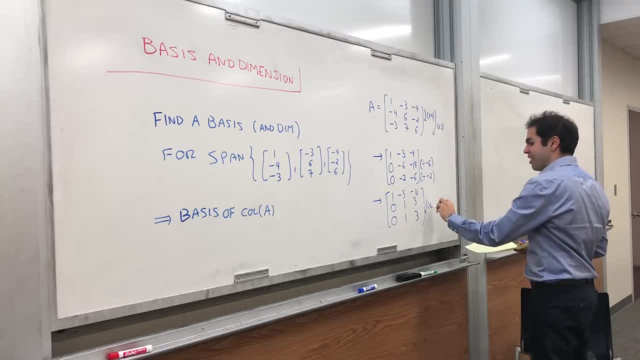 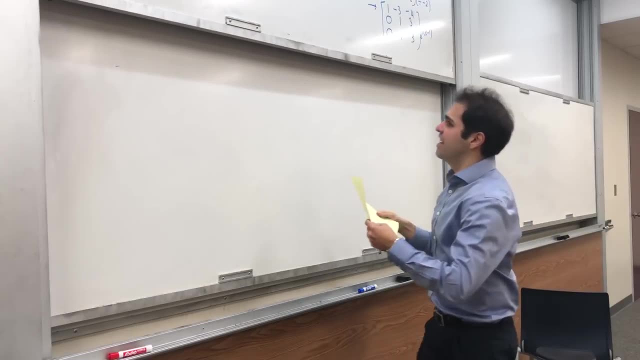 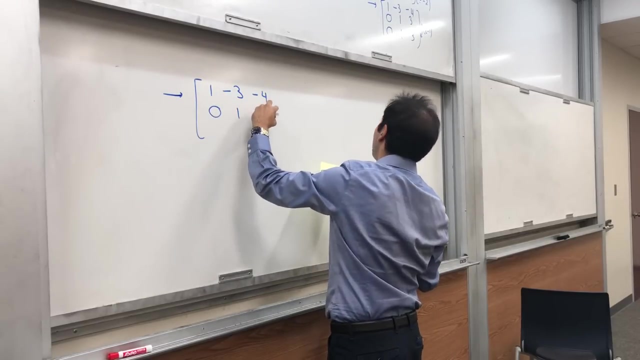 How nice. you can subtract the second row from the third And we get in the end 1 minus 3 minus 4, 0, 1, 4, sorry, 0, 1, 3, and 0, 0, 0.. 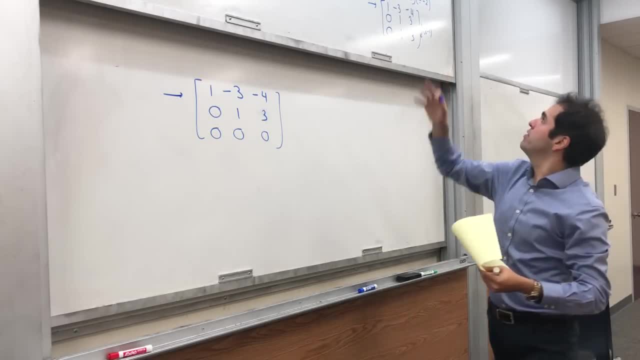 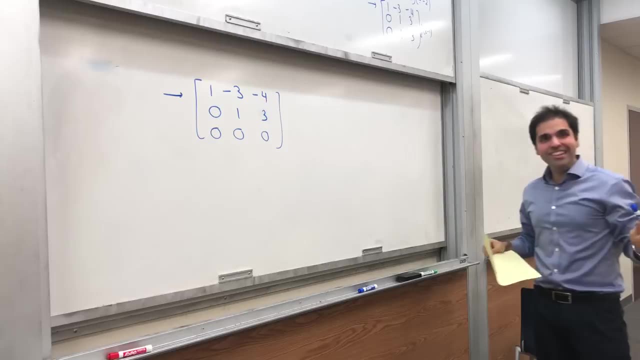 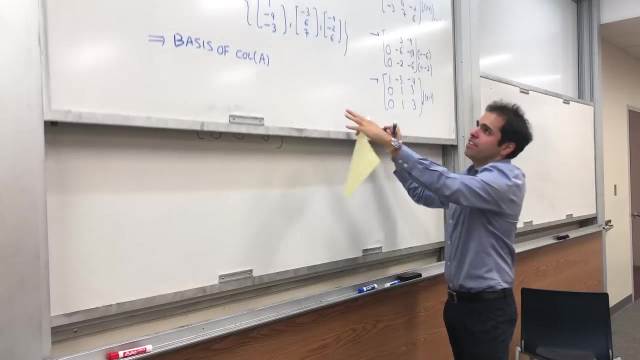 All right, and the question is: so maybe let me let me rewrite this. We had our matrix, or I'll show it to you. If you know linear algebra- which I hope by now you're better at it- to find a dimension of this space. it's the dimension of this column space which is the rank. 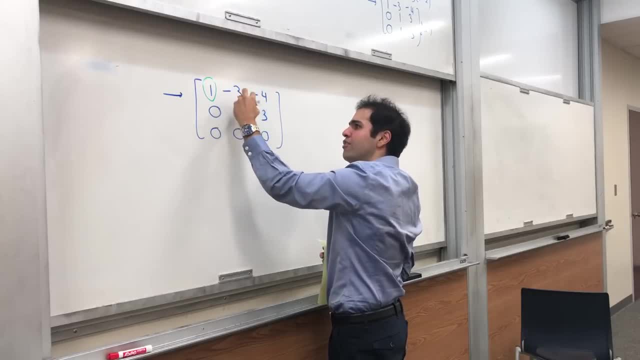 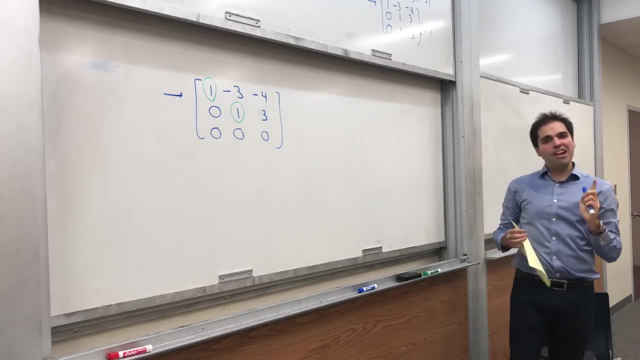 and which is the same as the number of pivots. So if you want a fast way of finding the dimension, you just count the pivots and you have 2.. But I don't think you can do that. I think it's very intuitive. so let's go back to, first of all, finding the basis for the column space. 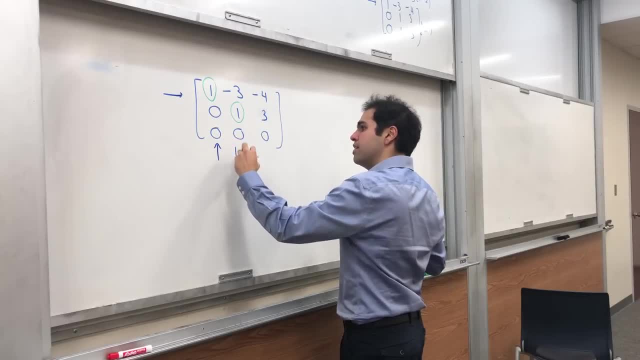 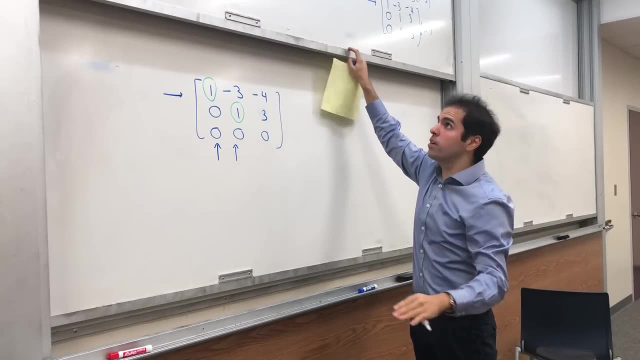 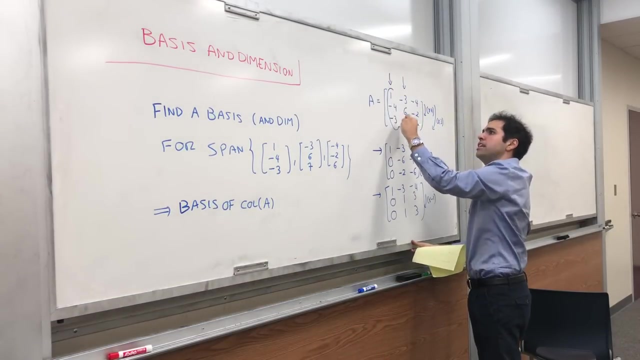 And remember what you do. You figure out the columns where the pivots are, which are the first and the second column And, very important, you have to go back to the first and second columns of A. So really a basis for your column space are those two vectors. 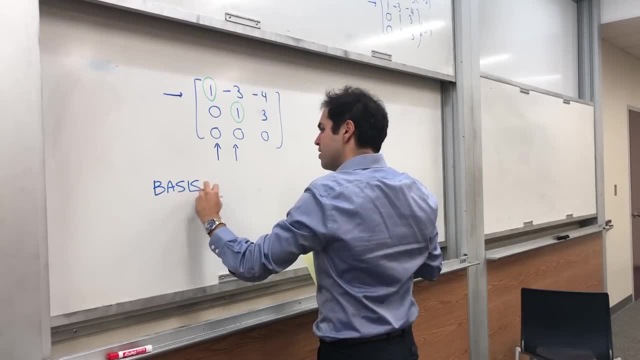 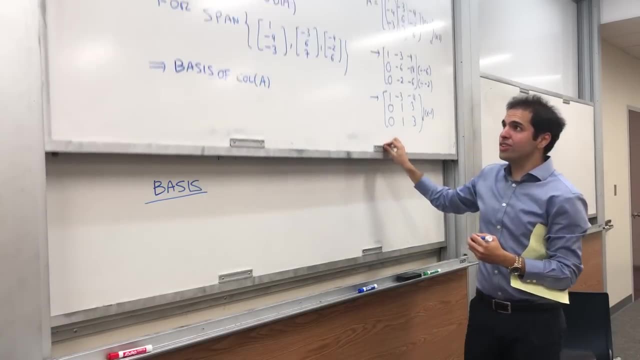 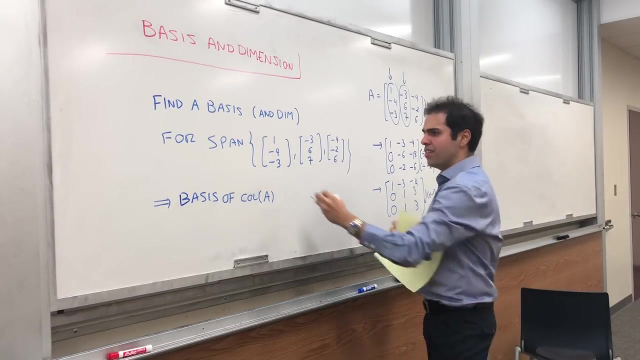 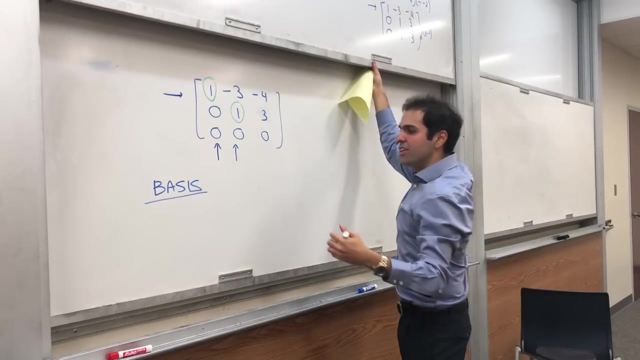 So basis is a cool thing. Not only a basis for the column space, but also a basis for your original space, because this is the same as the column space. In other words, to find the basis of your original space you do, you just pick the first two vectors here. 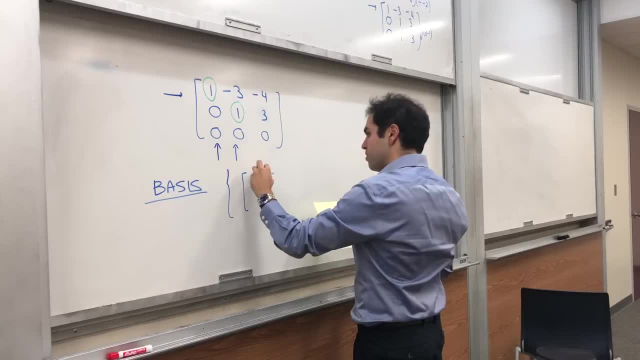 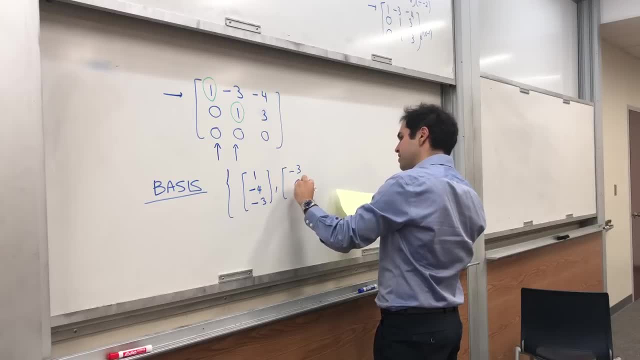 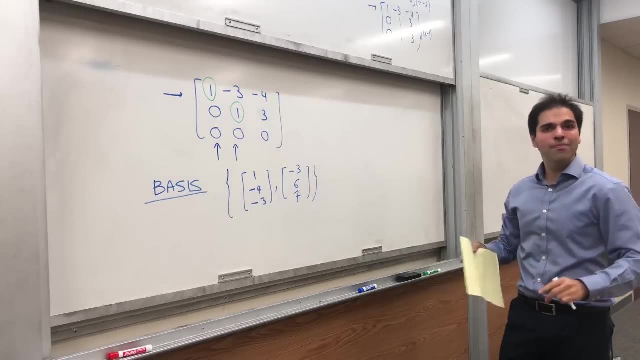 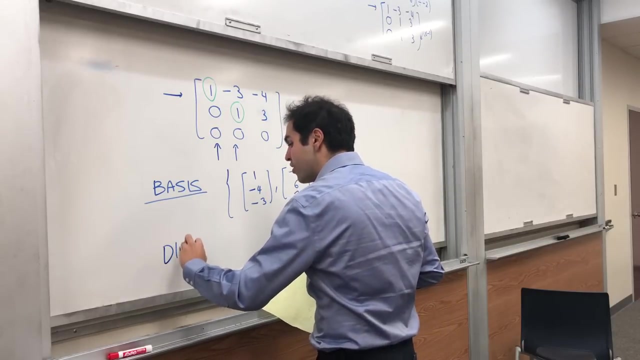 4 minus 3, and minus 3,, 6,, 7.. That's a basis. And then how do you find a dimension? Very easy: You just count the number of vectors in the basis, Because that is literally the definition of dimension. 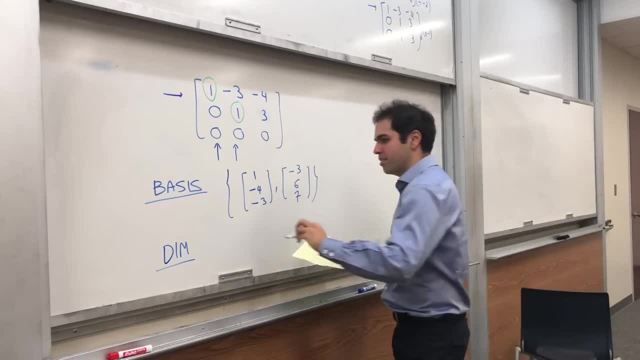 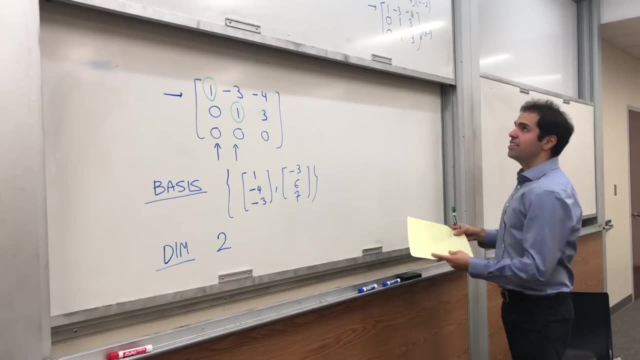 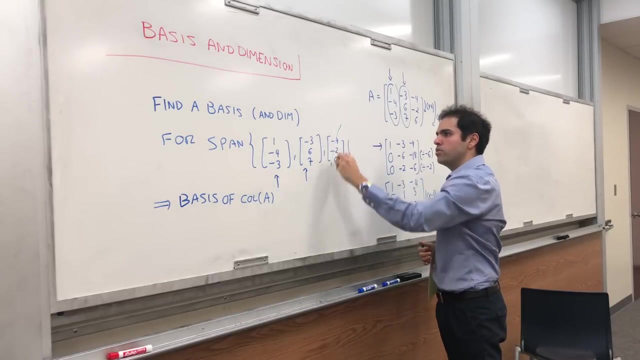 The number of vectors in any basis for your subspace. So dimension is then 2.. Now what is this saying? It says something very cool. It says not only that this vector is completely redundant. so it turns out you can write this vector as a linear combo of the other ones. 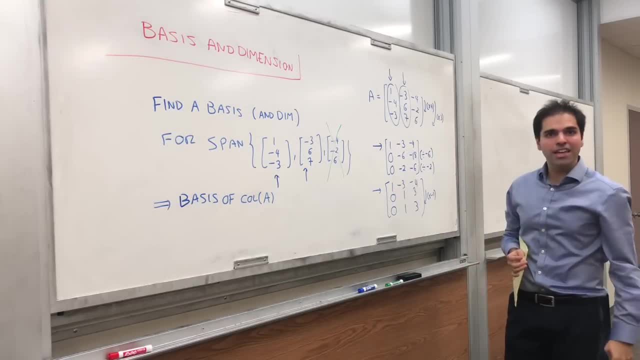 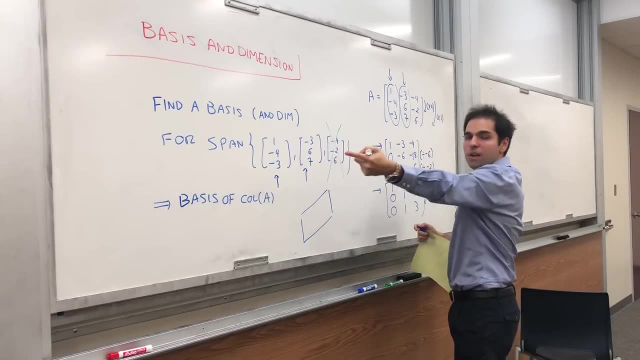 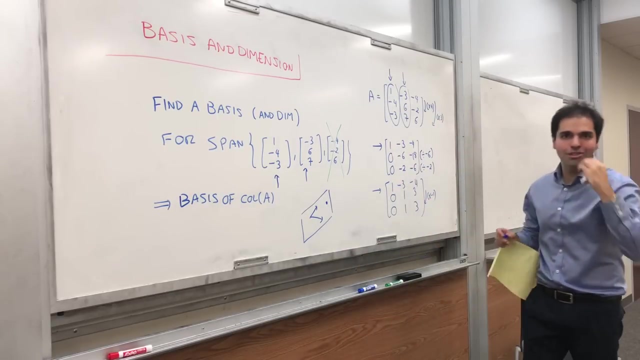 but also this thing that looks three-dimensional is actually two-dimensional. So if you want to draw it what it really is, it's a plane in R3 spanned by the first two vectors, Where the third one is just so vectorless, redundant.